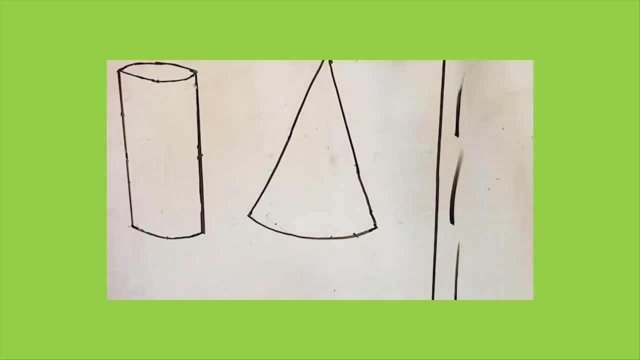 However, on non-Euclidean surfaces this is not true. On a cylinder, three different line shapes appear extrinsically. Horizontally, a line gains the shape of a circle. Vertically, it carries a regular linear shape And in any given diagonal direction a spiral may be formed. 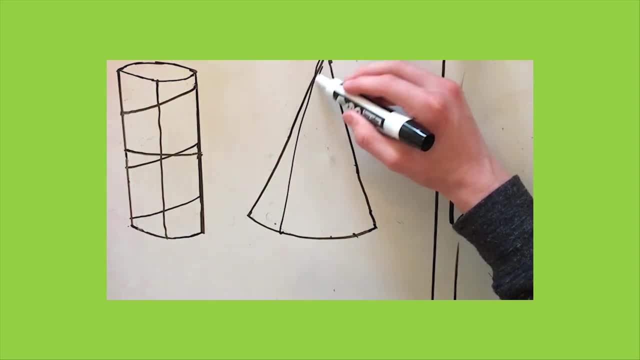 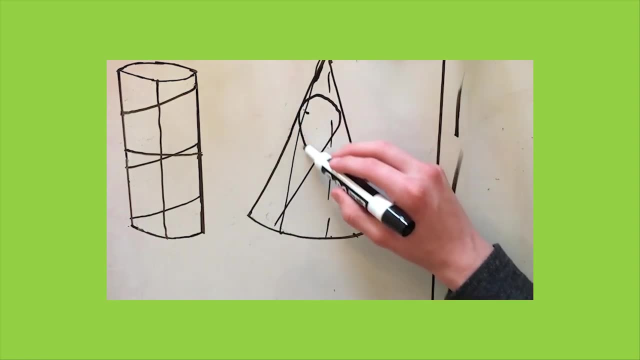 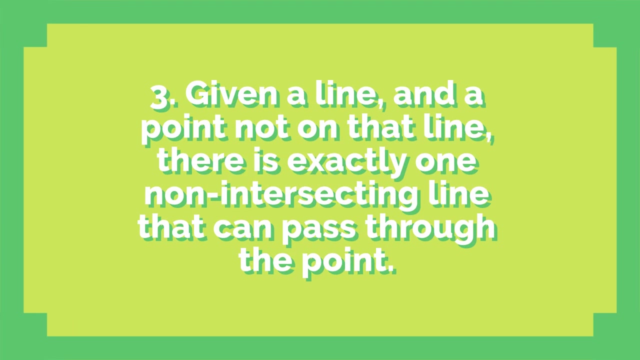 On a conical surface, two distinct lines appear. Vertically, a parabola is formed, And either horizontally or diagonally, a ribbon shape is formed. Another conclusion is that, Given a line and a point, not on that line, there is exactly one non-intersecting line that can pass through that point. 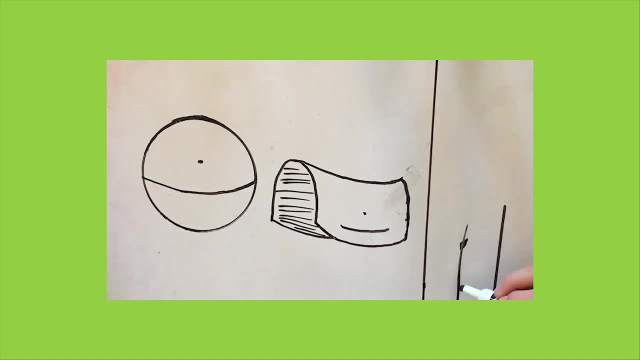 On two-dimensional surfaces this is true. There can only be one line that passes through a point that doesn't intersect that line. On a sphere, all lines must intersect each other, While on a hyperbolic surface, there can be infinite lines that do not intersect another line passing through a point. 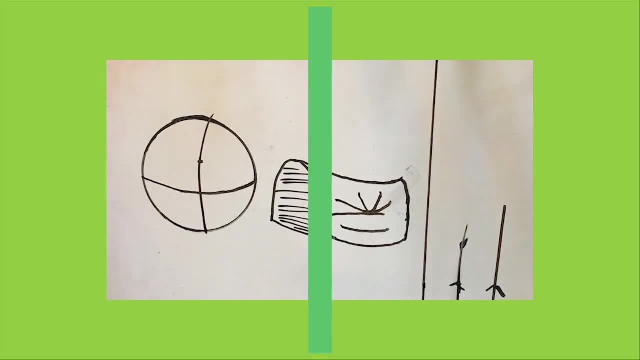 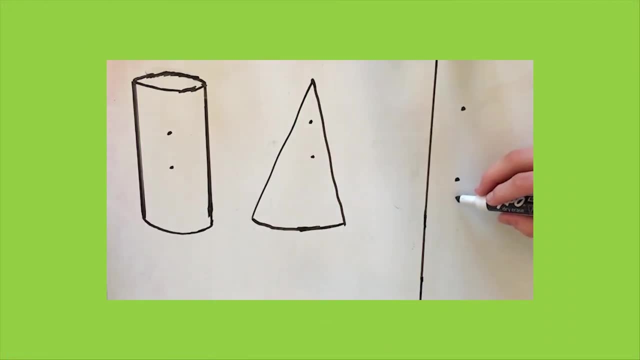 Therefore, the statement is false on these surfaces. The fourth conclusion is that two points determine a unique line. If there were two points on a Euclidean surface, only one line could be drawn. However, on cylinders and cones, this is not the case. 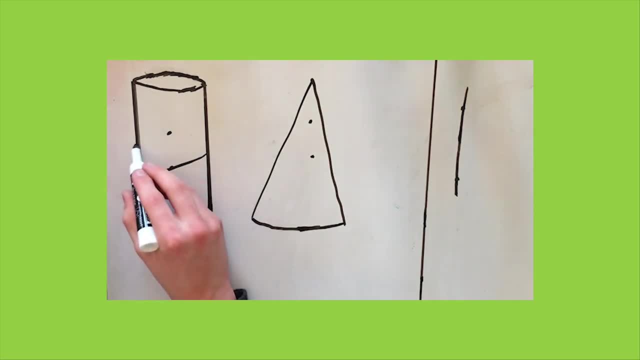 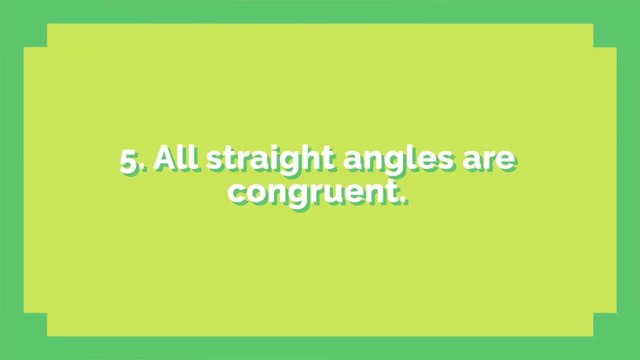 On a cylinder at two points, numerous spirals can be drawn And in some cases a singular straight line On a cone. two points may determine extrinsically a parabola and a ribbon or multiple ribbons. The fifth conclusion is that all straight angles are congruent. 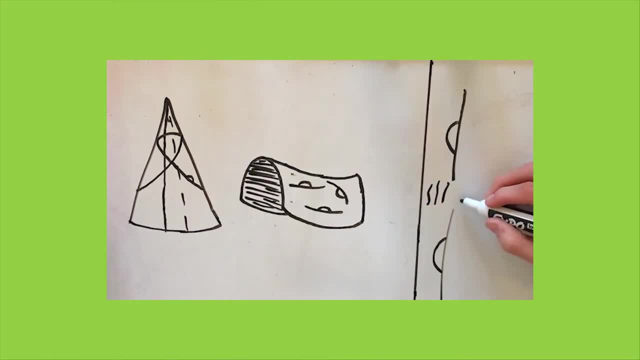 On a flat plane, this is true each measuring 180 degrees, Yet this is not true on conical and hyperbolic surfaces. On a cone, all lines not going through the point measure 180 degrees. However, a line going through the point will always measure less than that. 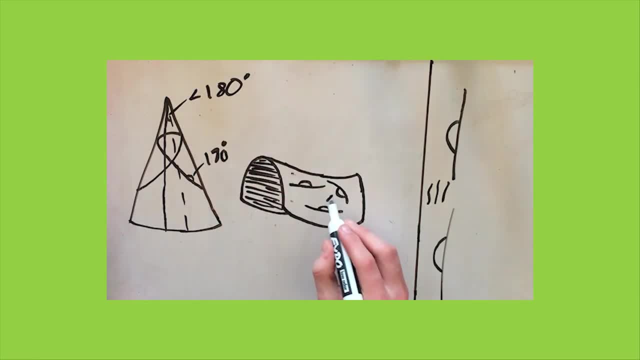 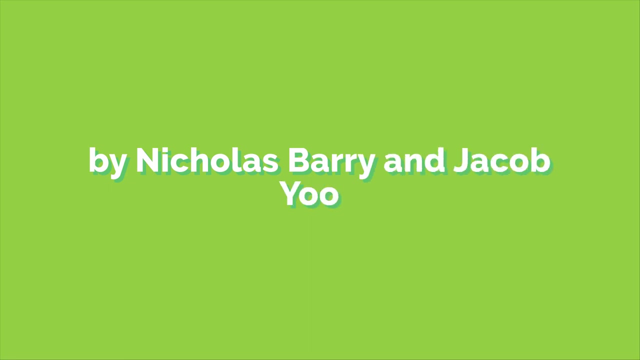 On hyperbolic surfaces, depending on where a line is drawn, the measure of a straight angle can change, being anywhere from greater than 0 degrees to less than 360 degrees. From all this we can gather that self-contained geometries can occur where not all Euclid's postulates apply. 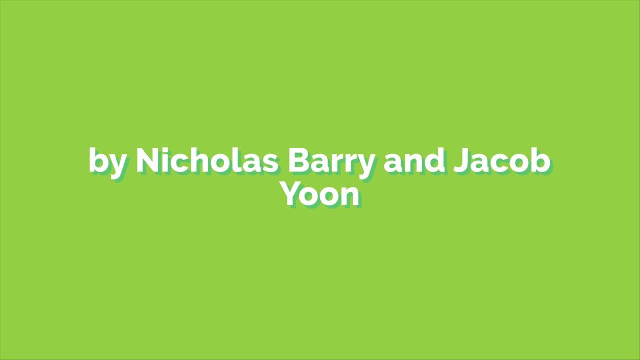 specifically curved surfaces. Subtitles by the Amaraorg community.